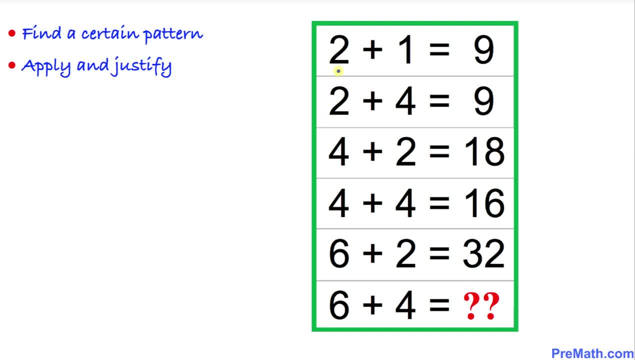 And now let's take a deep breath and start working on the very first numbers on the first row. Now let's focus on these two numbers: 2 plus 1.. If you add them, that's going to give us 3.. Now we are going to multiply by itself once again. 3 times 3 is going to be 9.. 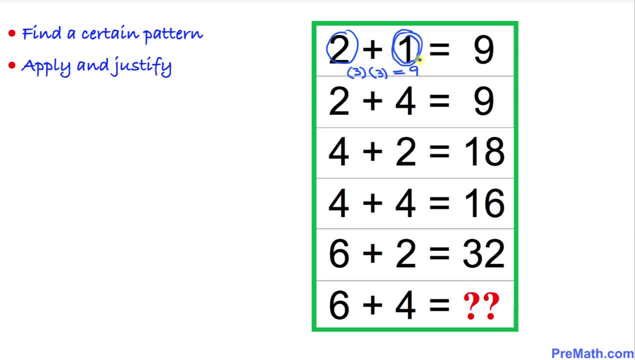 And then I'm going to divide by this second number: 9 divided by 1.. 1 is going to be 9.. Let's move on to our second row. Look at these two numbers: 2 plus 4 is going to give us 6.. And then I'm going to multiply 6 to itself. 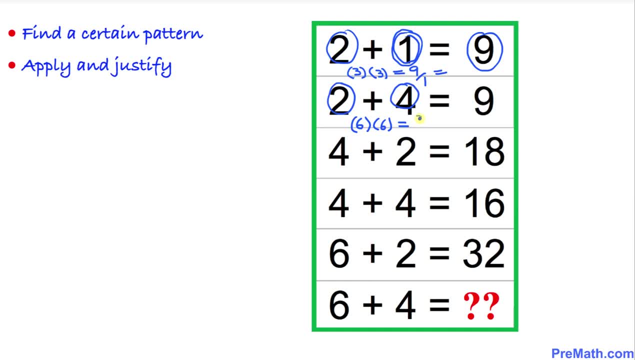 6 times 6 is going to be 36.. And then I am going to divide by this second number, this one, 4.. 36 divided by 4 is 9.. 36 divided by 4 is 9.. Likewise, let's do the same thing with this third row. 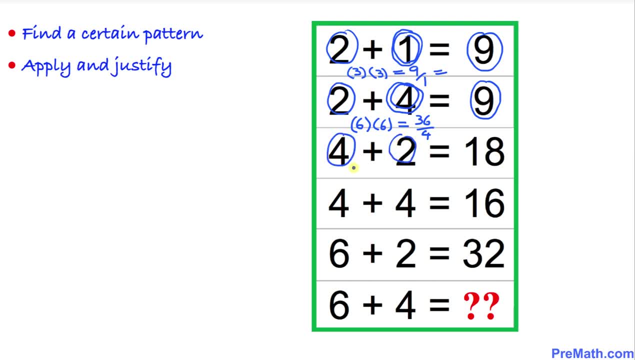 4 plus 2 is 6.. And then we're going to multiply 2 itself 6 times 6 is going to be 36.. And then we are going to divide by this second number, which is 2.. That is going to give us 18.. 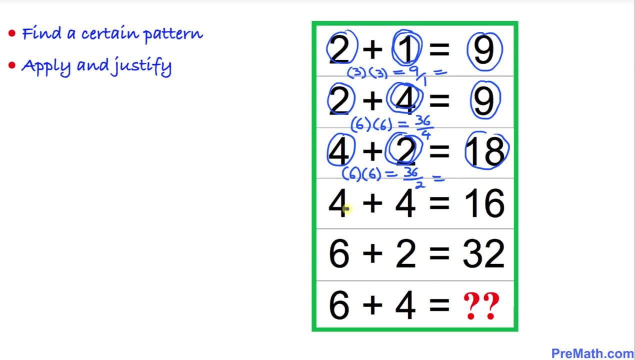 And now, next, the set of numbers 4 plus 4 is going to give us 8, isn't it? Now we are going to multiply 8 to itself. 8 times. 8 is 64 divided by 4, this number, the one, 4 at the bottom. 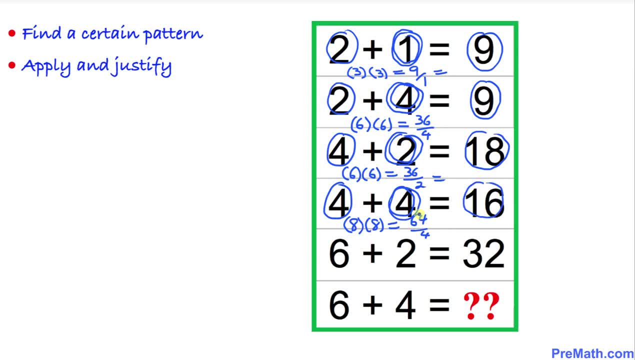 That is going to give us 16.. All right, so far, so good. Let's move on to this one now. Next numbers: 6 plus 2.. 2 is going to give us 8.. Let's go ahead and multiply 8 to itself. 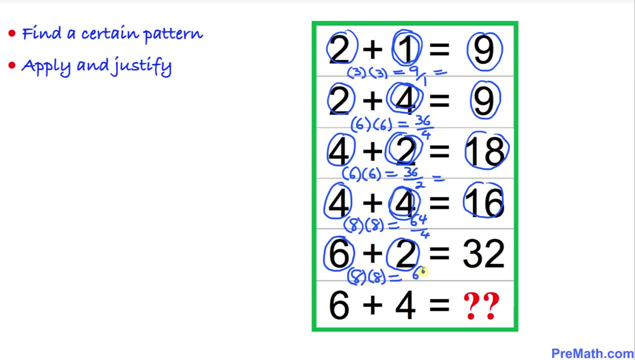 8 times 8 is going to be 64. And then, divided by this second number, which is 2,, divided by 2.. 64 divided by 2 is 32.. And finally, we are going to apply the same analogy on this: 6 and 4..